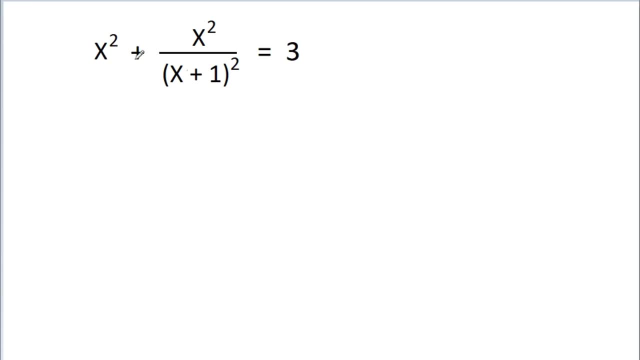 In this video we have given that x square plus x, square by x plus one whole square is equal to three and we have to find the value of x. So here we have given that x square plus x, square by x plus one whole square can be written as x by x plus one. 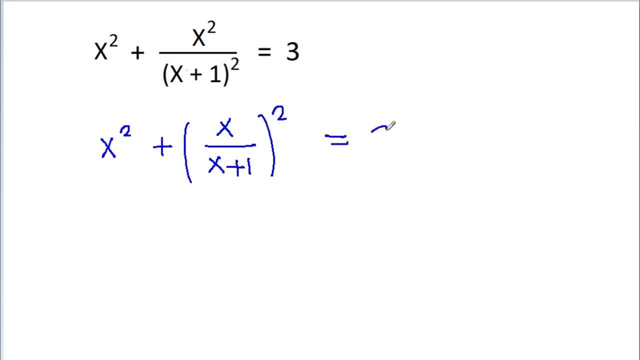 whole square is equal to three and now we can write this as x square plus here x to one in bottom. so we can write this: x plus one minus one by x to one whole square is equal to three, and now we can get x to the square plus x to the. 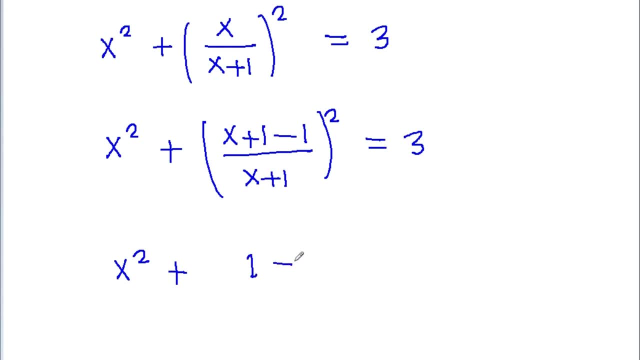 one minus to x to second plus dé to production in this, and we will write: 1 by x plus 1 will be 1 minus 1 by x plus 1. whole square is equal to 3 and now we can get x square plus. here we get 1 minus 1 by x plus 1, whole square minus 2. 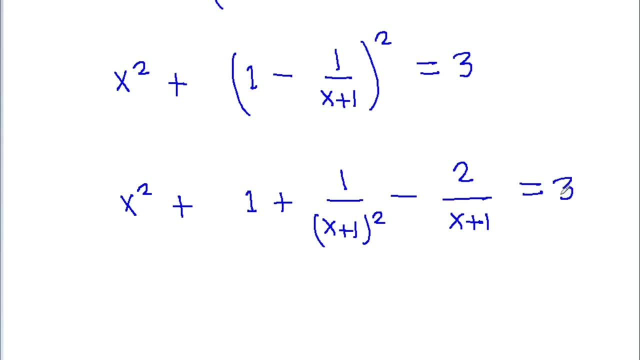 by x plus 1 is equal to 3, or it is x square plus 1 by x plus 1. whole square minus 1 minus 2 by x plus 1 is equal to 3, or x squared plus 1 by x plus 1. 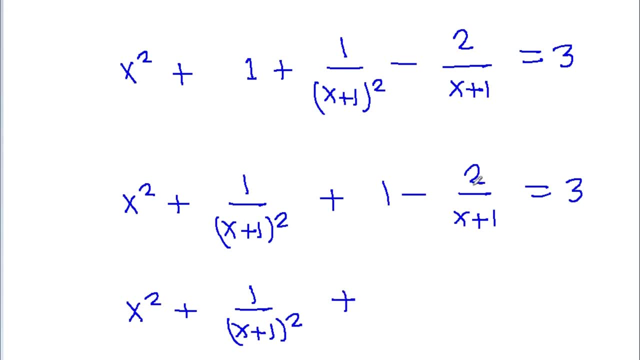 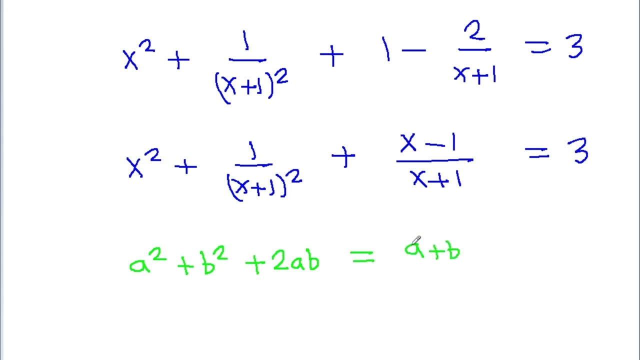 whole square, minus 1 minus 2 by x plus 1 will be X minus 1 by x plus 1. okay, equal to 3. and now we know that a square plus b square plus 2ab is equal to a plus b whole square. so we have x square 1 by x plus 1 whole square. so for 2ab, 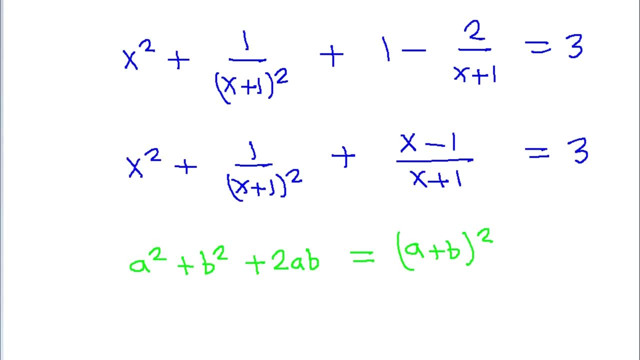 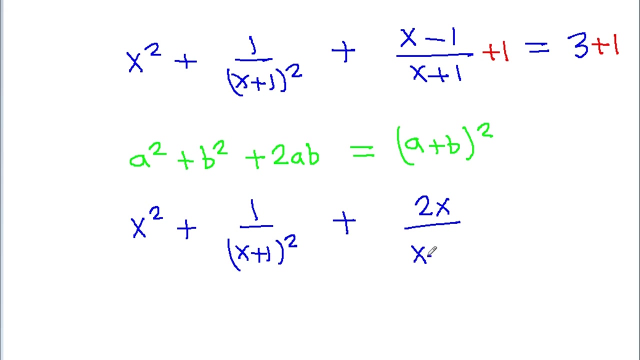 we need 2 x by x plus 1. so here, if we add on bot side so we can get here x square plus 1 by x plus 1, whole square minus x minus 1 plus x minus 1 will be 2. x by x plus 1 is equal to 3 plus 1 will be 4, and 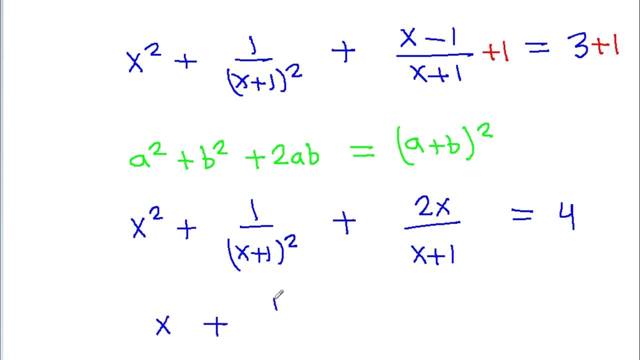 9. now we can get x plus 1. by x plus 1, whole square is equal to 4, or we can get x plus 1 by x plus 1 is equal to 2, or x plus 1 by x plus 1 is equal to minus 2, and 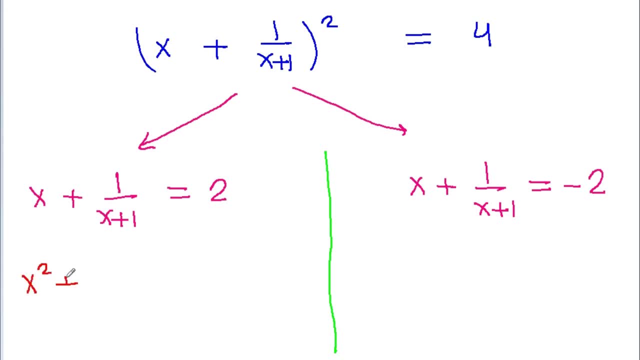 from here we can get x square plus x plus 1 is equal to 2 x plus 2. or we can get x square minus x minus 1 is equal to 0.. And from here we can get x is equal to minus b plus minus root. under b square minus 4 ac, that will be plus 4 by 2a. 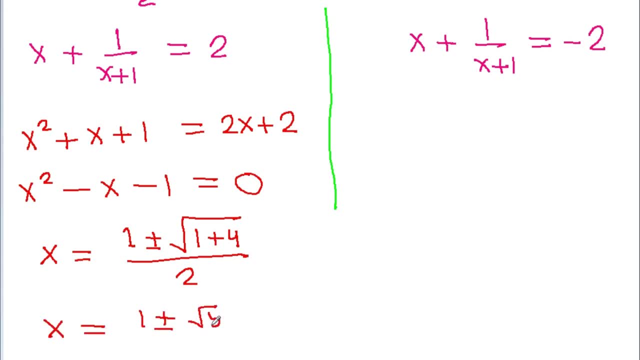 or x is equal to 2a, equal to 1 plus minus root 5 by 2, and from here we can get x square plus x plus 1 is equal to minus 2, x minus 2. or we can get x square plus 3, x plus 3 is equal to 0, or we can get x is equal to: 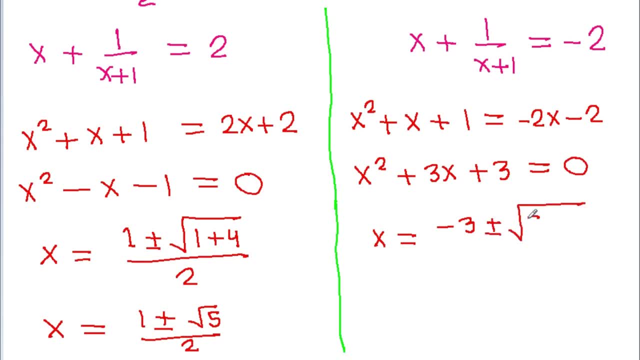 minus b plus minus root under b square minus 4ac, that will be 12 by 2a, that is 2. so we get: x is equal to minus 3 plus minus. i root 3 by 2. so these are the four values of x: two real values and two complex values. you.